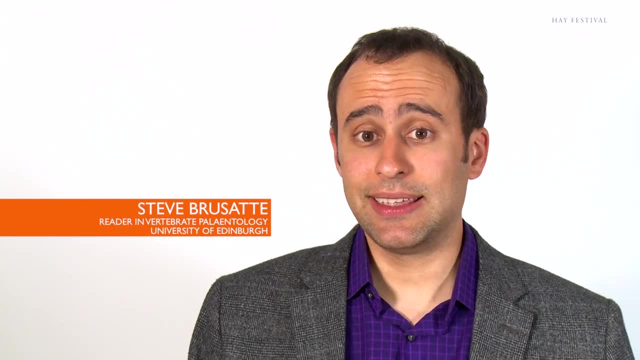 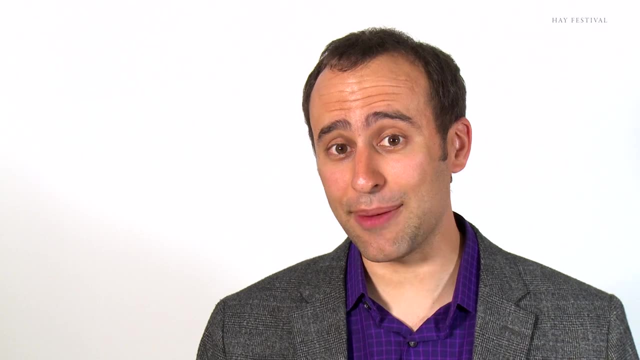 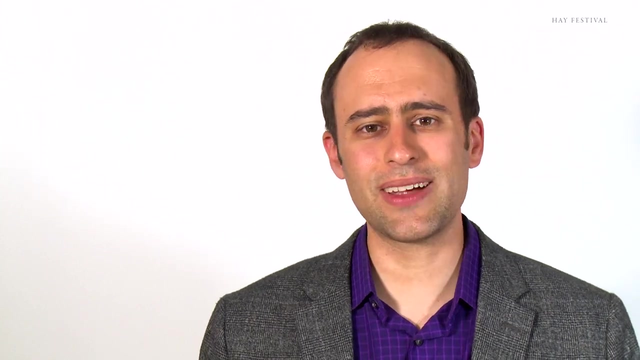 I'm a paleontologist and that means I study fossils: Fossils to understand how the Earth has changed over time, how evolution works, And fossils- whether it's a bone or a tooth, or a leaf or a footprint, whatever it is, these fossils are clues to lost worlds. They're 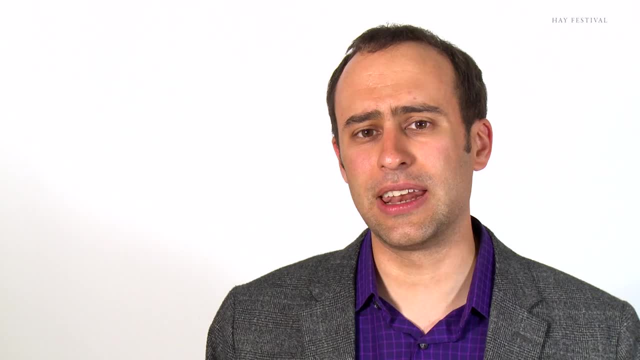 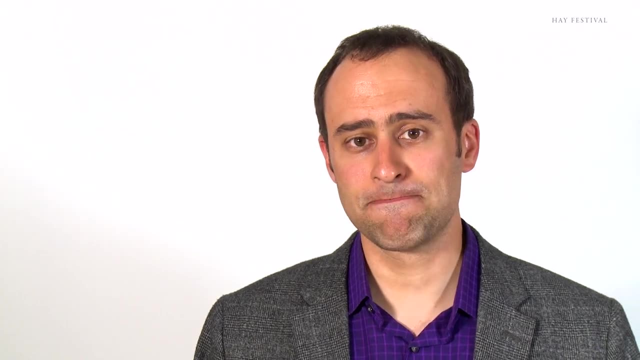 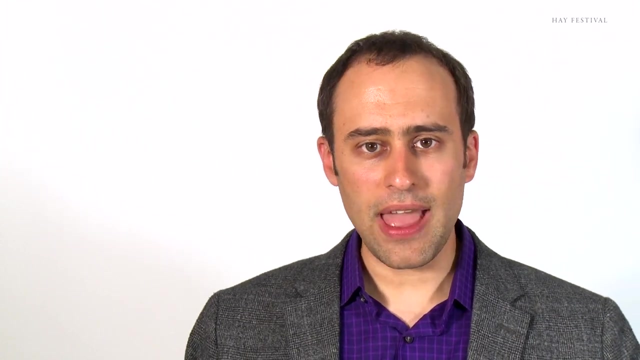 clues to the history of our planet, the long history of our planet, because Earth is four and a half billion years old And fossils tell that story. And one of the things that fossils tell us is that sometimes, occasionally, rarely, there are these events called mass extinctions. And these are moments in time very brief. 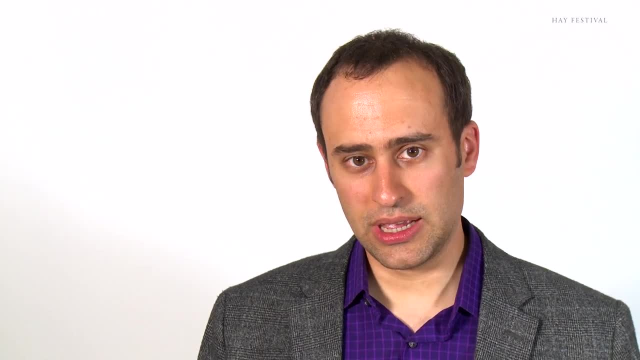 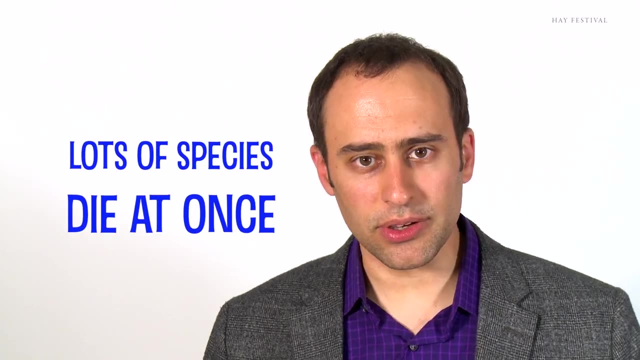 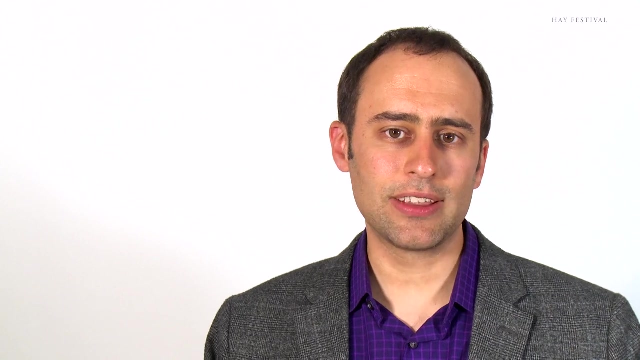 periods of time where, all around the world, lots and lots and lots of different plants and animals die out together all at once because of some kind of single mass extinction. And some mass extinctions have been caused by glaciers, by an ice age, Others have been 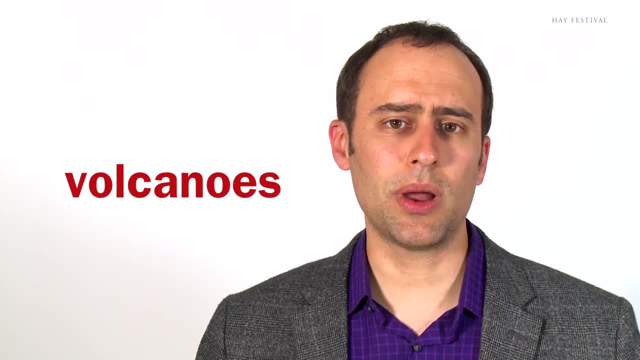 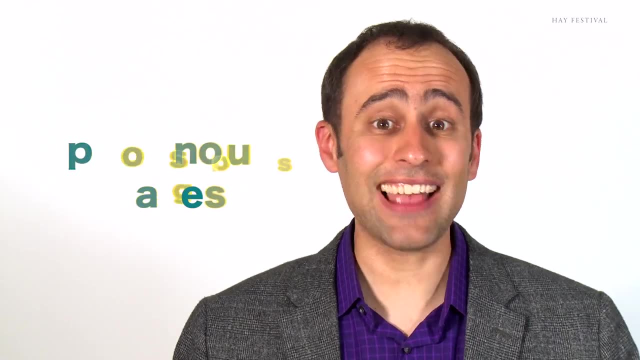 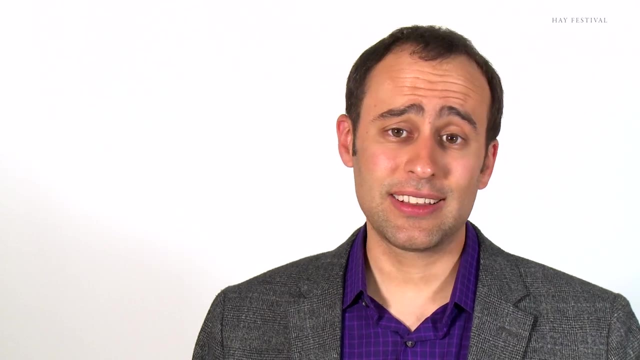 caused by volcanoes, by big eruptions, eruptions that bring lava, of course, and scar a lot of the Earth's surface, but also bring with them a lot of poisonous gases that go up into the atmosphere- carbon dioxide, methane- these things that cause global warming And other. 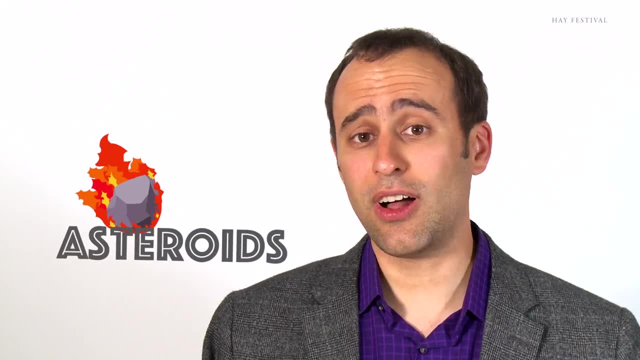 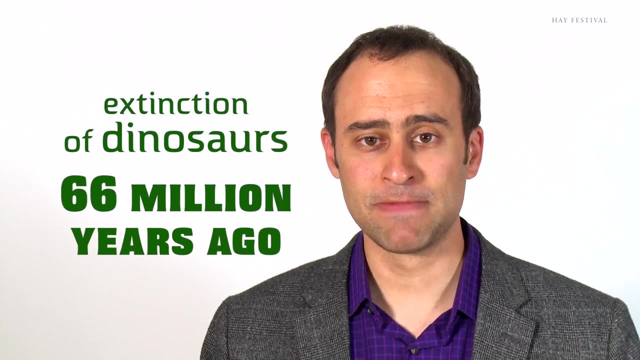 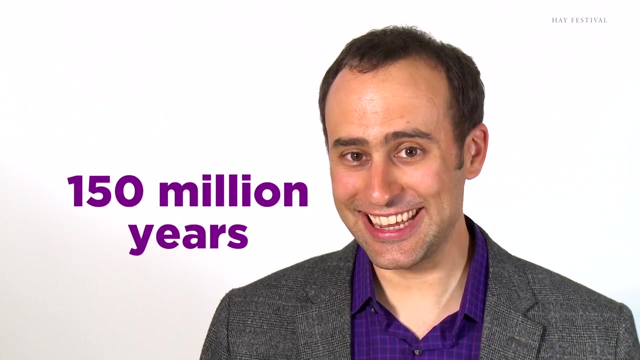 extinctions have been caused by asteroids. The most famous one of all, of course, is the one that killed off the dinosaurs 66 million years ago. This is the extinction everybody knows about, And it was due to an asteroid. The dinosaurs had been around for 150 million. 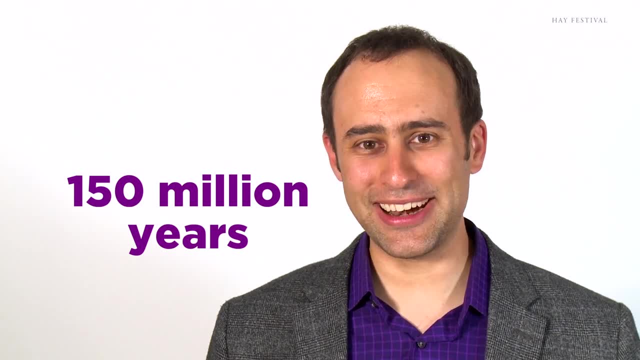 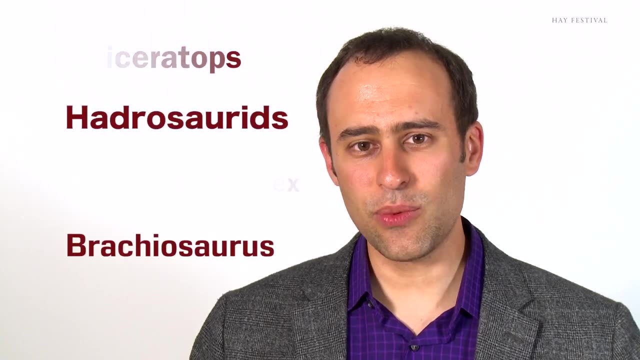 years. They were a global empire. They were dominant animals. You had your T rexes and your triceratops and your long necked dinosaurs and your duck-billed dinosaurs, And they were on top of their game until one day, literally one day. 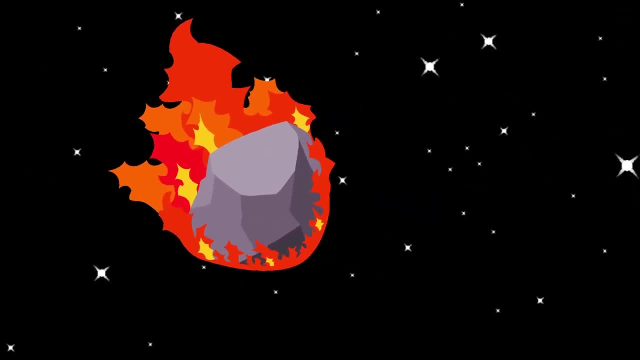 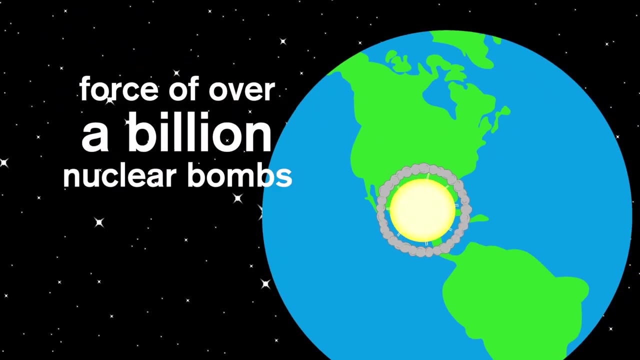 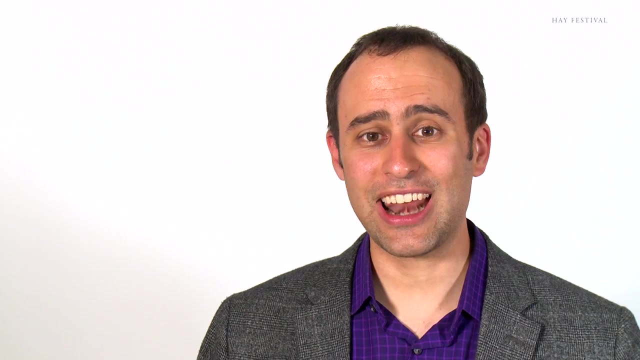 A six mile wide asteroid came crashing down. It was traveling faster than a jet plane. It smashed into the Earth with the force of over a billion nuclear bombs. It punched a hole in the crust that was over 100 miles wide And that caused destruction Instantaneously.